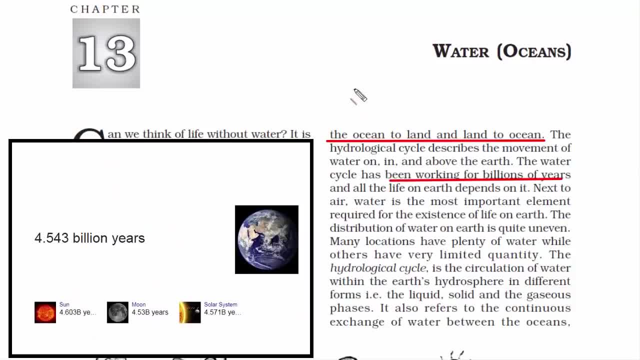 happening for billions of years, because the earth is estimated to be 4.5 billion years old. Hence the water cycle has been working for billions of years And basically now it has become the most important element for the existence of life on earth. And if this cycle doesn't continue, then 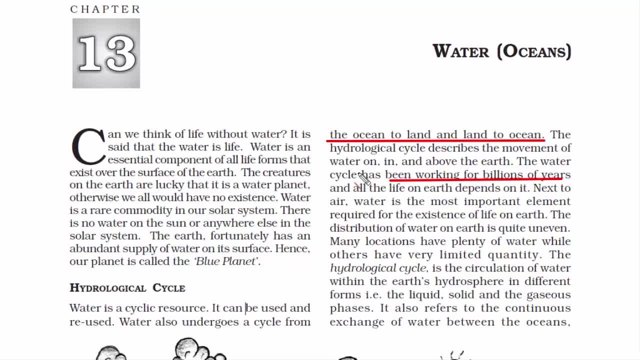 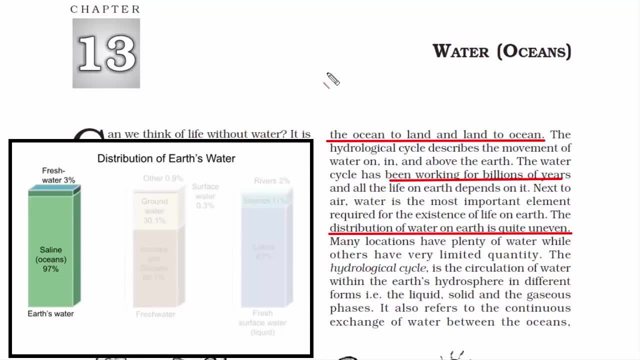 earth will not get sufficient water, And that can be detrimental to all the living beings on earth. So here it says: the distribution of water on earth is quite uneven. What we mean by that is, only 3% of water is fresh and the remaining 97% is ocean water, And ocean water is extremely salty. 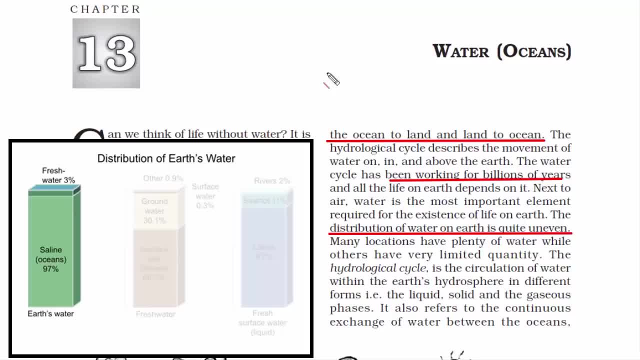 Human body only needs a small amount of salt And that makes the ocean water not fit for consumption. And if you look at the 3% of fresh water that exists on earth, in that 69% is found in glaciers, Then 30% is the underground fresh water that we extract with the help of borewells. 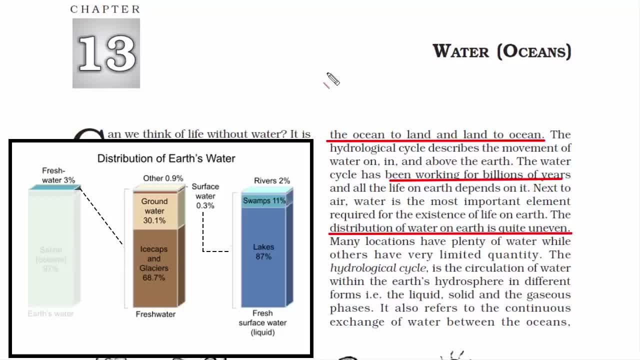 And the remaining less than 1% of fresh water is located in lakes, rivers and swamps, And another important aspect here is that many places on earth have plenty of water, while others have very limited quantity If you look at the statistic. this is what makes water a rare commodity, and it is also highly exploited. 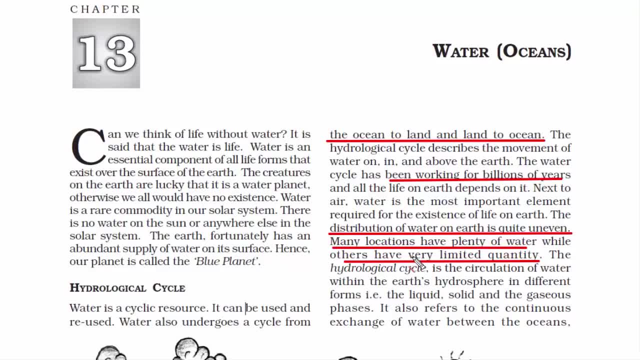 Moments back I told you about the water cycle. So water cycle and hydrological cycle is the same. So basically, in this cycle the circulation of water within the earth's hydrosphere is in the form of liquid, solid and gas. 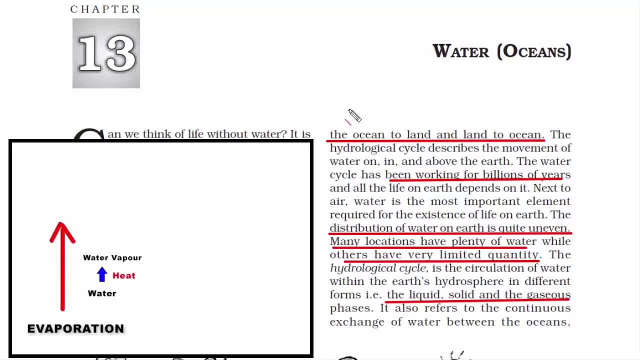 Now, evaporation is the process by which water is converted into water vapor, which is in gaseous state, with the help of heat. After evaporation, condensation takes place. In condensation, water vapor turns into liquid or solid, depending on how low the temperature is. 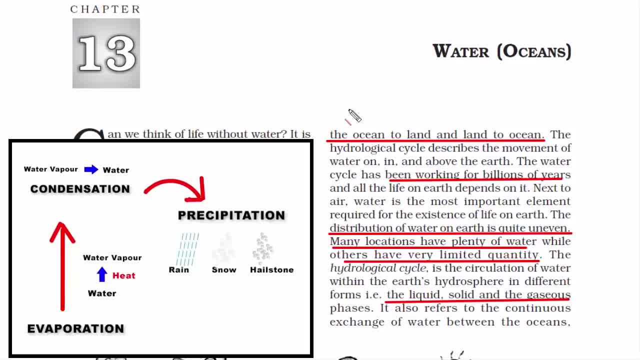 After condensation, precipitation takes place. Now, precipitation occurs both in the form of rainfall, snow and ice pellets. If it is rain, then it is in liquid state, and if it is snow and ice pellets, then it is in solid state. 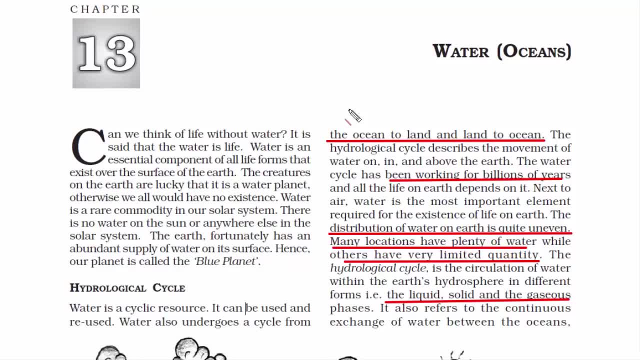 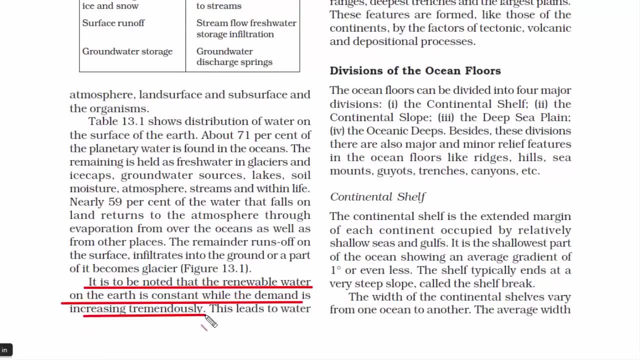 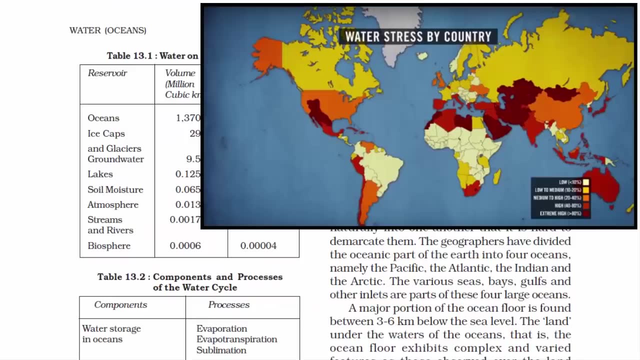 So this is how water circulates within the earth's hydrosphere. The renewable water on the earth is constant, while the demand is increasing tremendously. Now this leads to crisis in different parts of the world. Have a look at this world map. You can see the countries currently dealing with extreme water scarcity. 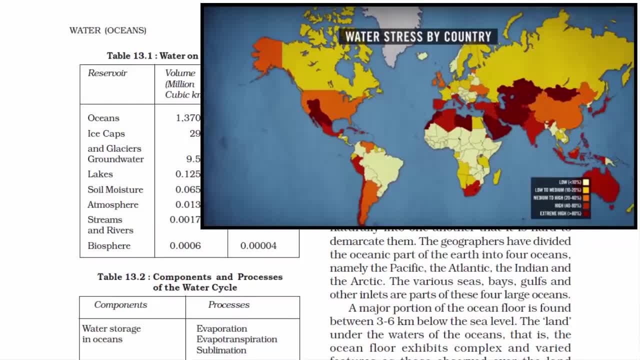 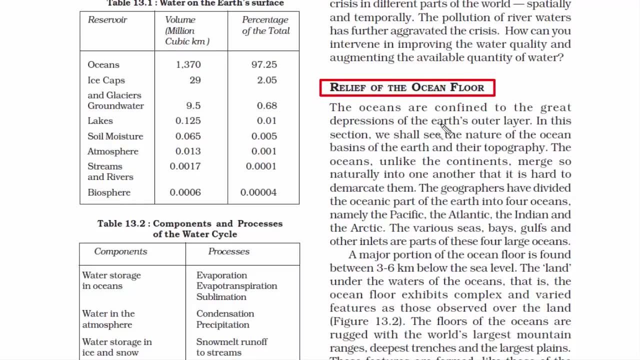 Dark color represents the country with extreme shortage of water. Pause the video and have a look at it. Let's go to the next topic: relief of the ocean floor. Now, when we say relief in geography, it means the topography of an area. 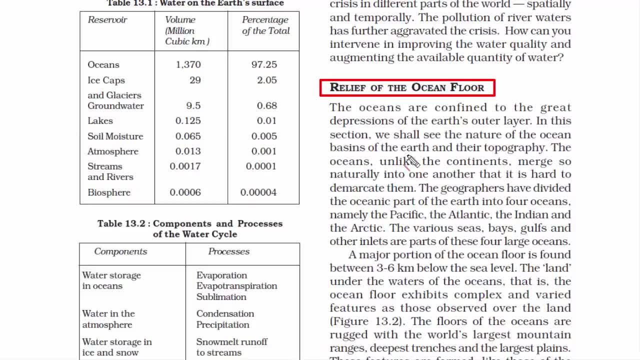 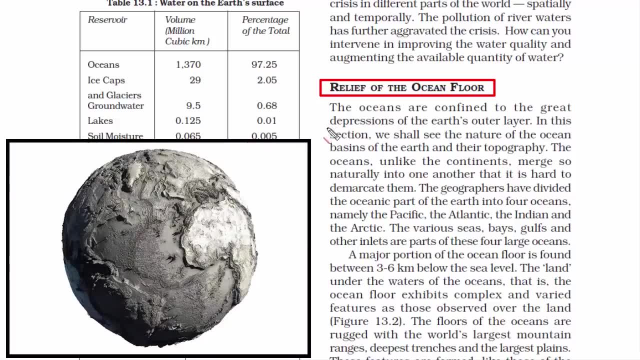 So relief of the ocean floor means the topography of the ocean floor. If you take a model of planet Earth and start digging in wherever you want to, wherever you are able to create a depression on the outer layer of the earth, that is where oceans are formed. 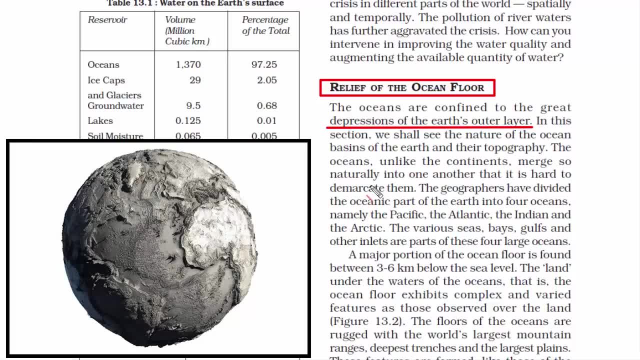 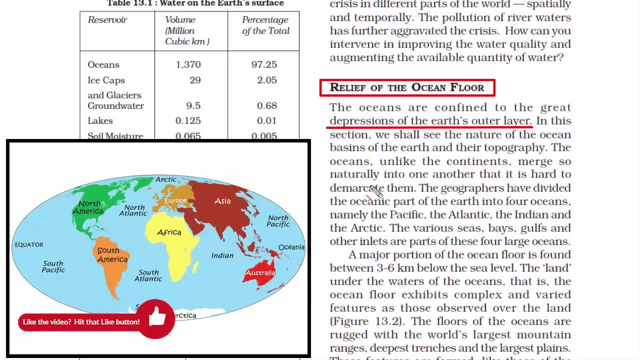 So basically, oceans are the great depression of the earth's outer layer. Wherever there is a depression, water gets accumulated, right. That's how oceans are formed. If you look at the world map, you will notice that the continents are not necessarily merged with each other. 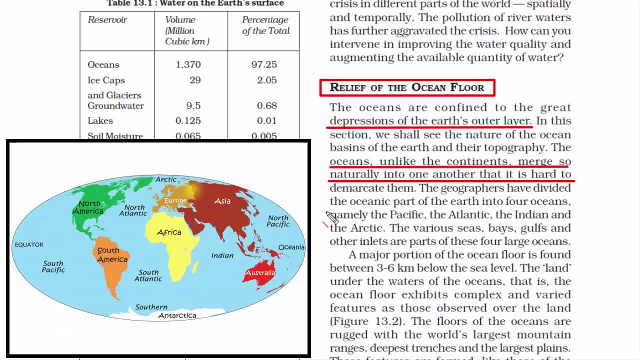 I mean, with an exception of Europe and Asia, they merge with each other. However, if you look at North America, Europe, Australia, Africa, South America, Antarctica, they don't merge with each other, But when it comes to oceans, they merge naturally into one another. 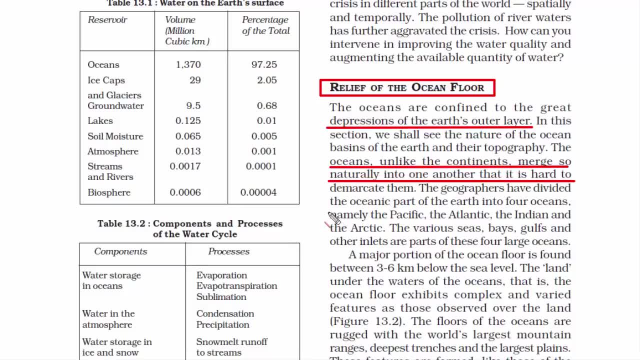 That means oceans of the world are connected with each other. We cannot create a boundary and say this is part of Atlantic and the other part is Pacific Ocean, But still for the studying purpose, geographers have divided the oceanic part of the earth into four oceans. 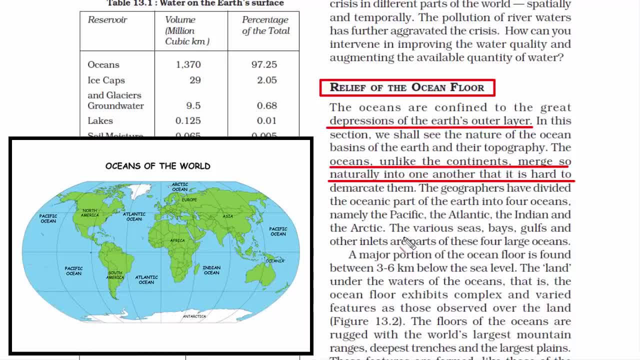 They are Pacific, Atlantic, Indian and Arctic. The various seas, bays, gulfs and other inlets are part of these four large oceans. The various seas, bays, gulfs and other inlets are part of these four large oceans. 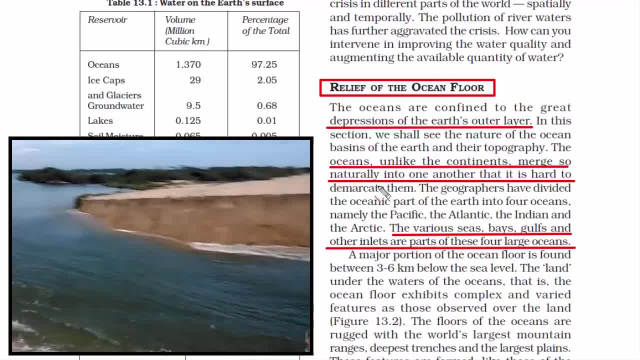 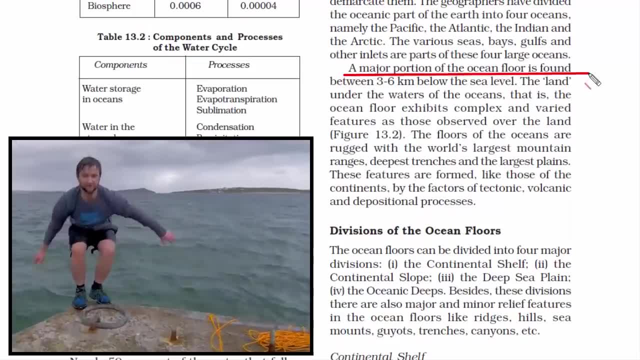 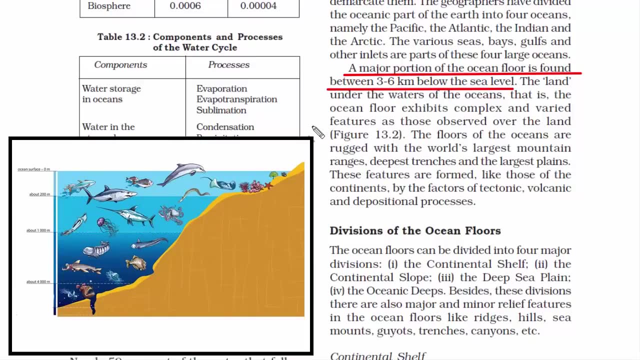 The various seas, bays, gulfs and other inlets are part of these four large oceans Because, ultimately, all the rivers, inland waterways, everything falls into a sea and sea is very much part of ocean. If you get an opportunity to jump in an ocean, you see that the major portion of the ocean floor is found between three to six kilometer from the sea level. 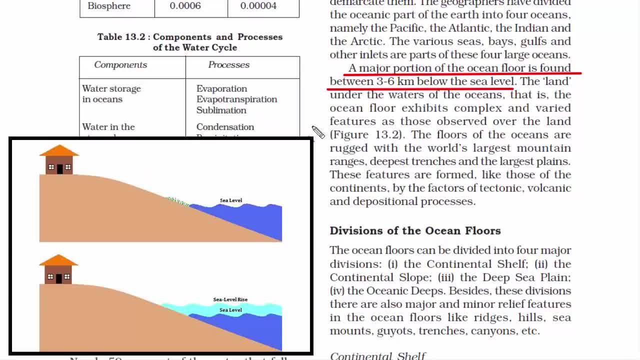 Now, sea level and ocean floor are two different things. A sea level is the level of the sea surface. Once you are at the sea level, you need to go three to six kilometer below in order to reach the ocean floor. Once you are at the sea level, you need to go three to six kilometer below in order to reach the ocean floor. 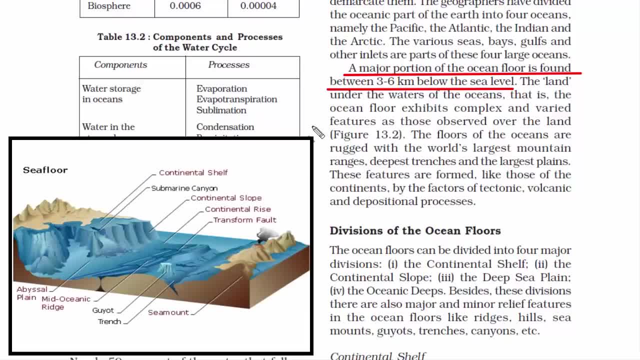 Once you are at the bottom of the ocean floor, the land under the water has exact, similar physiographic features, like how we see outside on a landmass. Once you are at the bottom of the ocean floor, the land under the water has exact, similar physiographic features, like how we see outside on a landmass. 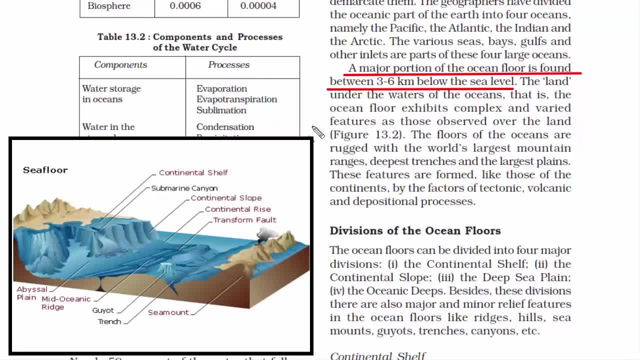 Once you are at the bottom of the ocean floor, the land under the water has exact, similar physiographic features, like how we see outside on a landmass. Once you are at the bottom of the ocean floor, the land under the water has exact, similar physiographic features, like how we see outside on a landmass. 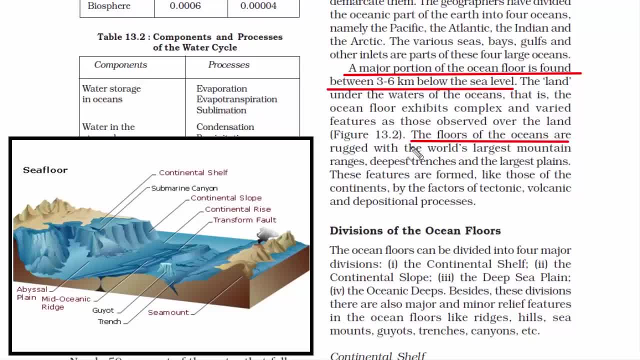 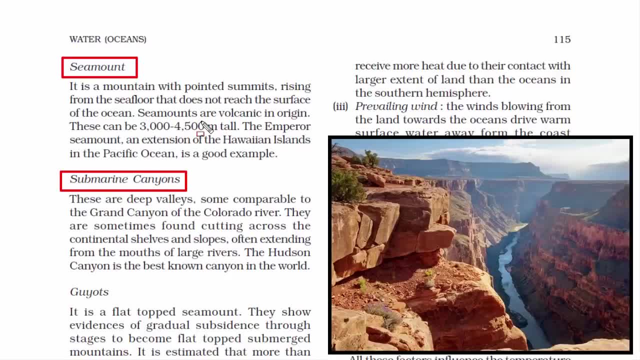 Submarine Canyons. When you hear the word canyon, it means a deep, narrow valley with steep sides. It is typically formed due to weathering and erosion activity done by rivers. They are often called as v shaped valley Because the stream of the river is so strong that it cuts the entire valley into a deep 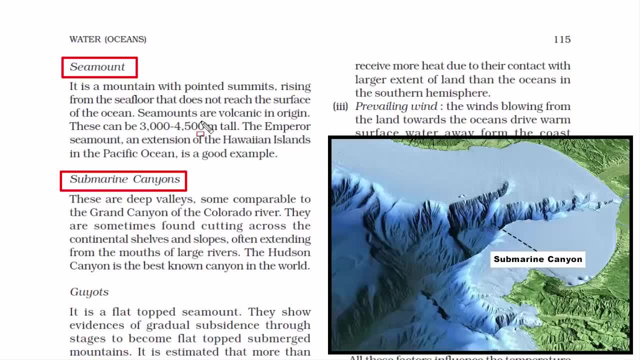 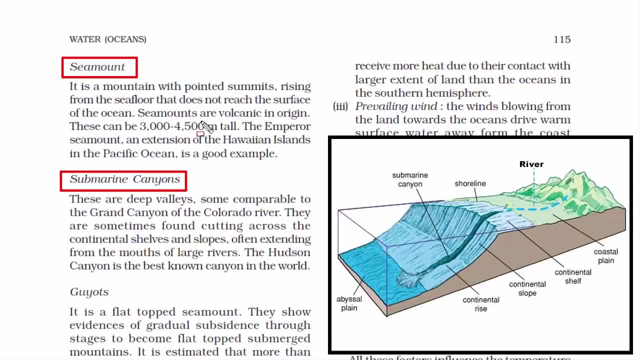 narrow valley with steep sides. Submarine canyons are formed at the junction between continental shelf and continental slope. Submarine canyons are formed at the junction between continental shelf and continental slope into the sea. these rivers bring massive amount of sediments, The water pressure. 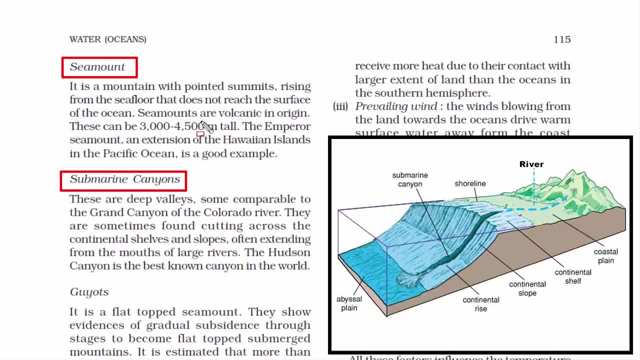 of a river can cut deep into a seabed by creating a deep, narrow channel called as canyons, And that's how submarine canyons are formed. Because of their complex topographic features, submarine canyons are considered major reservoirs of 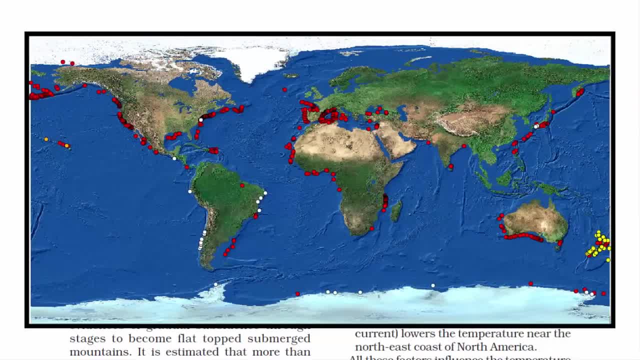 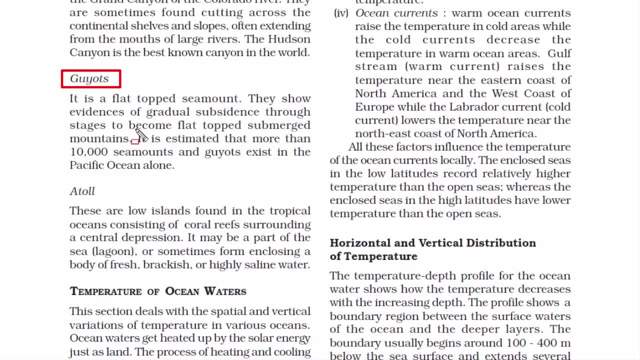 marine biodiversity. Have a look at this picture. In this picture you can see the global distribution of submarine canyons. The fourth minor ocean relief feature is Gyo. Now this term is pronounced as Gyo. Gyo is an undersea mountain. 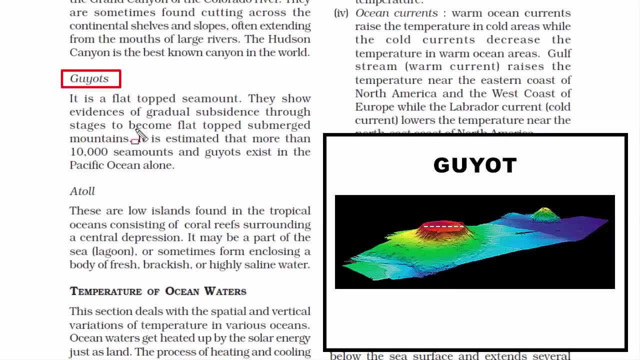 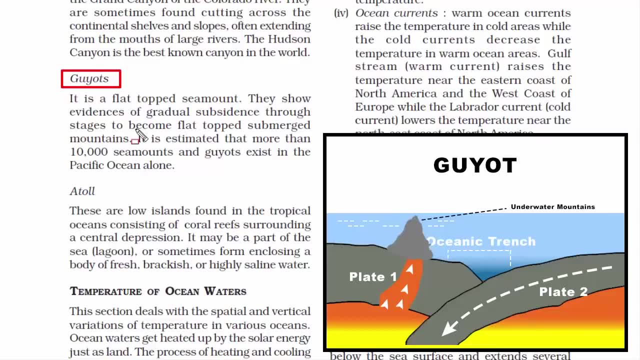 basically a seamount with a flat top, Since it is a type of a mountain, hence it has to be of volcanic origin. Volcanic activity forms all kinds of underwater mountains. Gyo are usually found in deep ocean basins. The reason: 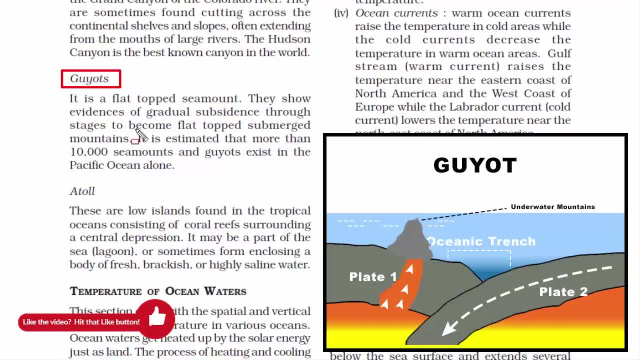 the top portion of the mountain is flat is because erosion by waves destroyed the top of the seamount, resulting in a flattened shape. Gyo are usually found in deep ocean basins. The reason the top portion of the mountain is flat is because erosion by waves destroy the top of the seamount, resulting in a flattened shape. Gyo are usually found in deep ocean basins. The reason the top portion of the mountain is flat is because erosion by waves destroy the top of the seamount, resulting in a flattened shape. Gheos are most commonly found in Pacific Ocean. 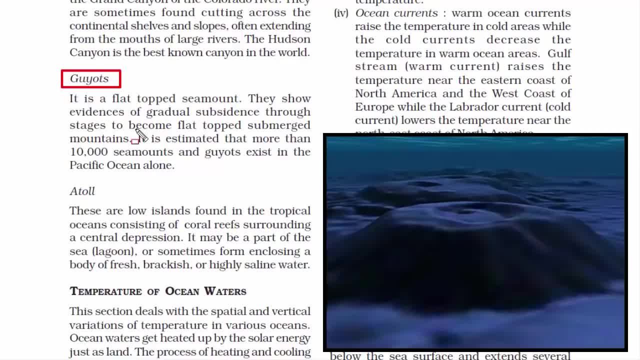 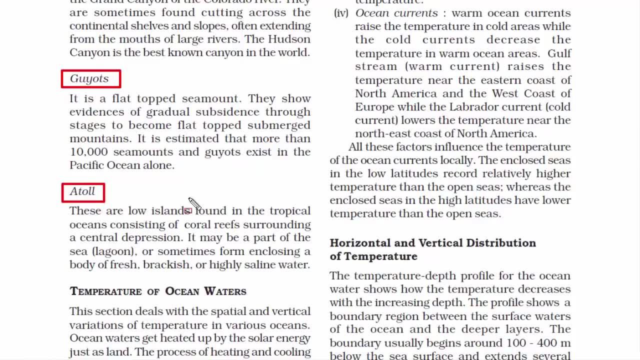 These gheos stand at least 3000 feet above the sea floor and the diameter of the flat top is at least 660 feet. The fifth and the last minor relief feature of the ocean floor is atoll. These are low islands found in the tropical oceans, consisting of caudal reefs surrounding. 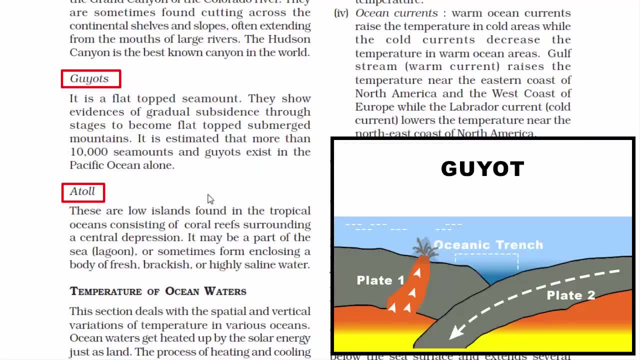 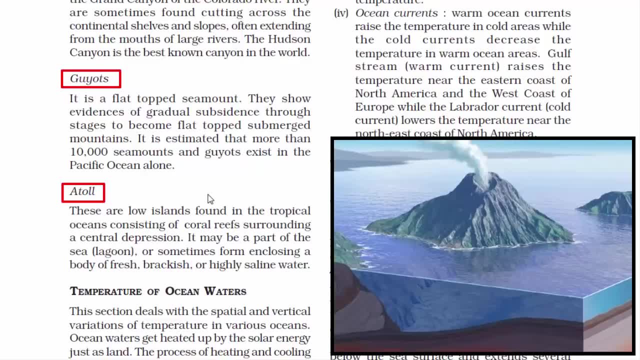 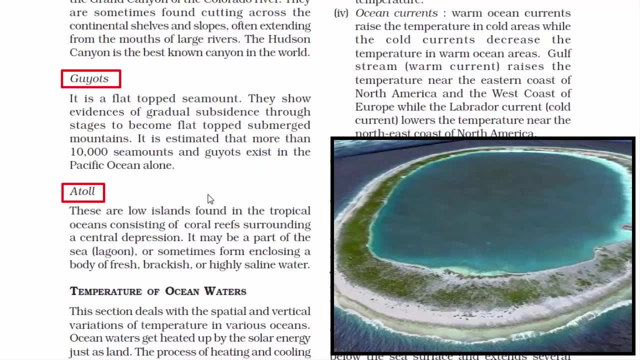 a central depression. So basically, when an underwater mountain is formed due to volcanic eruption, it pierces the surface of the ocean. As time passes, a caudal reef is formed around the volcanic island or the sea mountain. As more and more time passes, the volcanic island sinks due to the erosive activities. 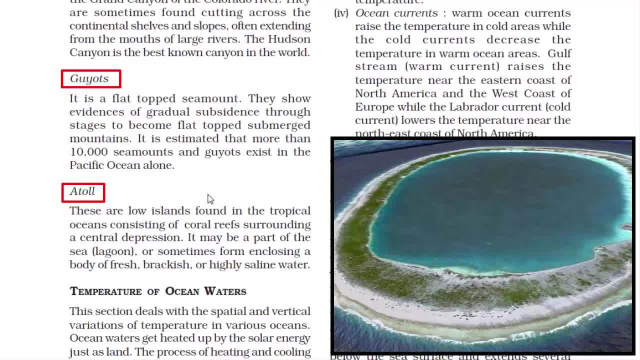 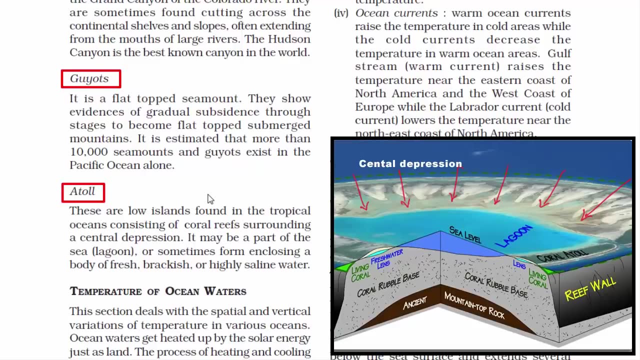 of the ocean wave making the top layer of the mountain flat, And in the previous topic we saw that they are called gheos. Finally, when the volcanic island completely sinks, all that is left is the surrounding caudal reef, And in between the caudal reef a lagoon is formed. 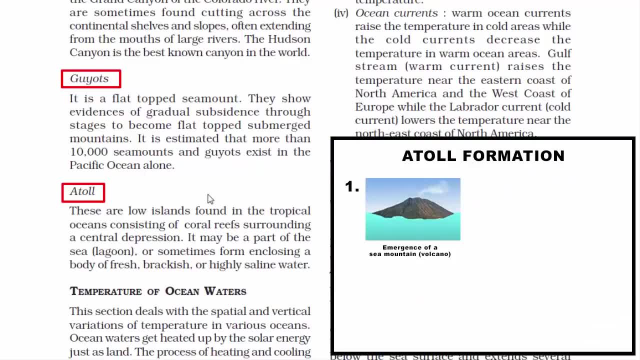 It's basically a central depression area. It may or may not be a part of the sea. If it is a part of the sea, then it will be highly saline, And if it is not a part of the sea, then it is a body of fresh, slightly salty water. 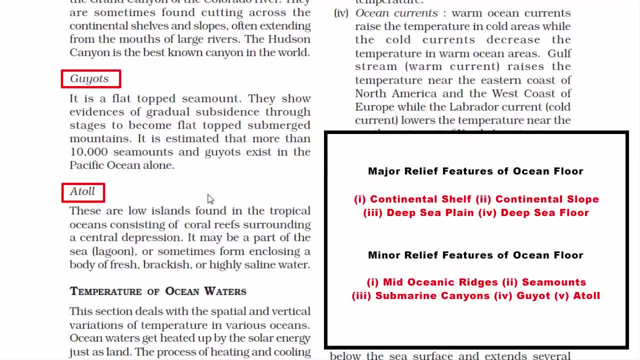 So these were some of the minor relief features of the ocean floor. We have covered both major as well as minor features of the ocean floor. If you have any doubt, please go through it again, because these features are very important from examination point of view, and if there's something that you don't understand, let 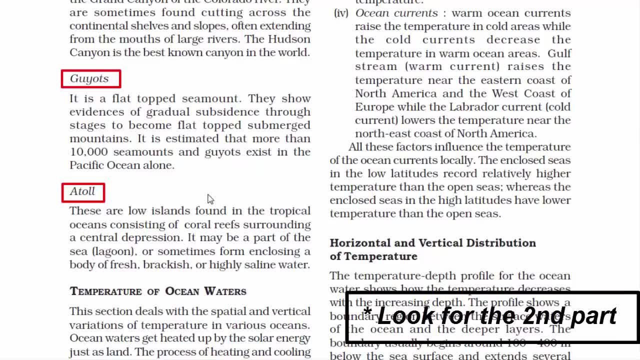 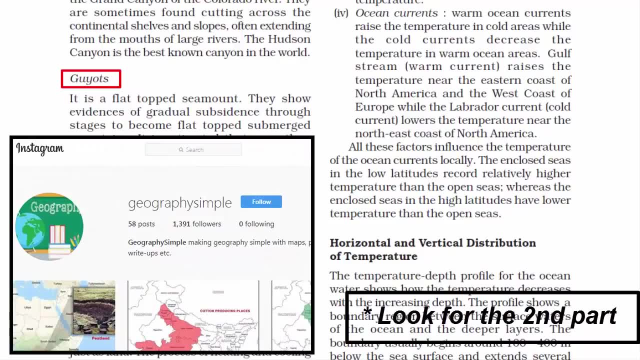 me know in the comment section There's also a second part to this chapter. that concludes the rest of the chapter. Make sure you watch it. Meanwhile, all the pictures and illustrations are available on the Instagram page of this channel. The link is there in the description.